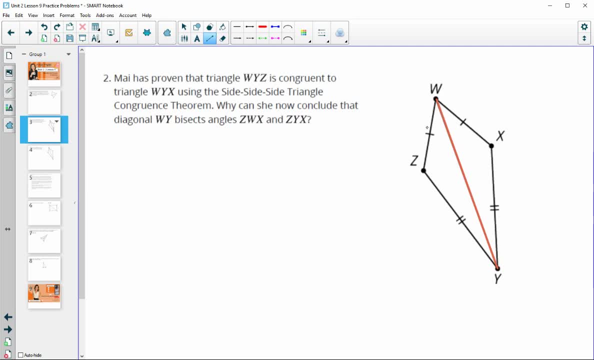 is the angle bisector of both ZY, sorry, ZWX and ZYX. So we can say: since the triangles are congruent, we know that ZWY, so angle ZWY is congruent to angle XWY because they are corresponding angles in congruent. 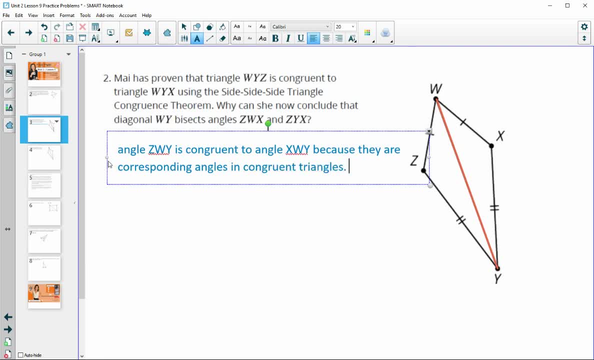 triangles And therefore WY would be the bisector of angle ZWX by definition. So the definition of a bisector is that it splits an angle into two congruent parts. So if we've got congruent angles, then we've got a bisector. So this segment is the bisector of this. 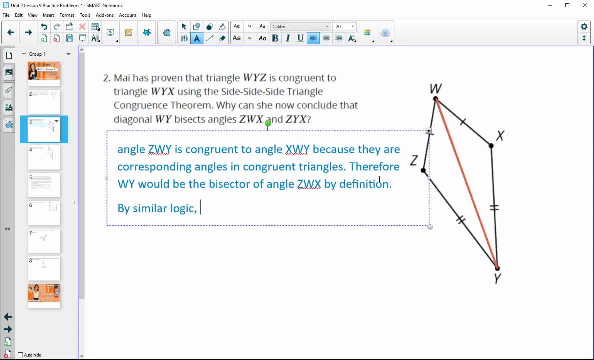 angle. So if we have a bisector of angle ZWX, then we've got a bisector of angle ZWX. So if we have a bisector of angle ZWX, you'd say that angle is a bisector of angle ZWY. 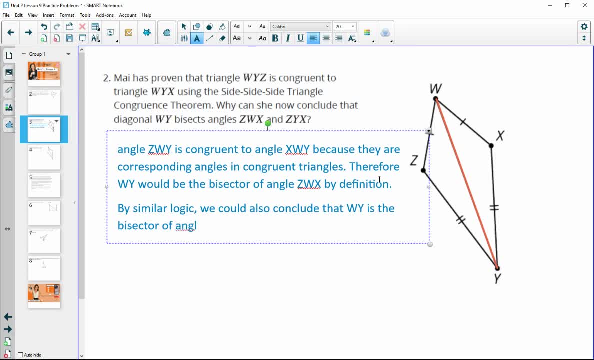 With this kind of simple logic, we can conclude that WY is the bisector of angle ZYX. can we say So? we would know that these two angles are corresponding angles and then they're congruent, since the triangles are congruent, which creates that bisector. 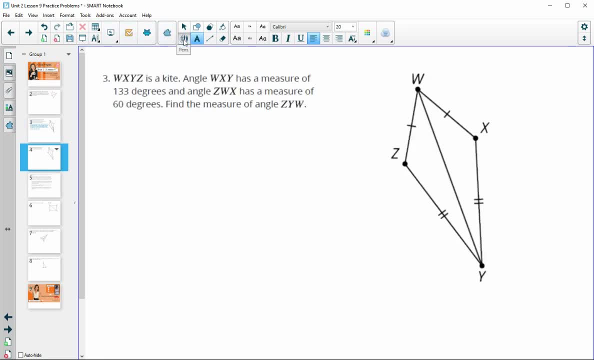 Okay, three is another kite, and this time it is giving us some angle measures. so angle WXY, so WXY, here is 133 degrees. and then it says that angle ZWX, so ZWX, this angle here is 60 degrees. and then it asks us to find the measure of ZYW. so 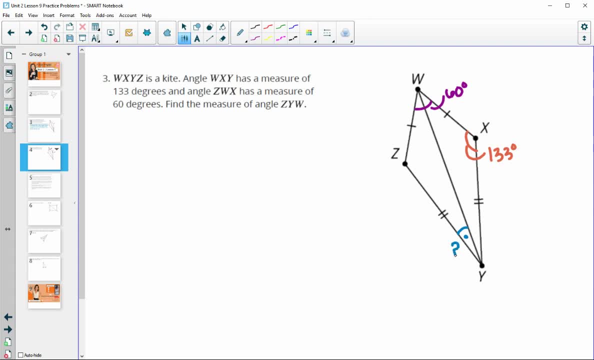 this little angle in here is what we're looking for. So, since we know it's a kite, we can see that this diagonal splits it into two congruent triangles, because this middle segment would be the same in both. and then we've got these other two. 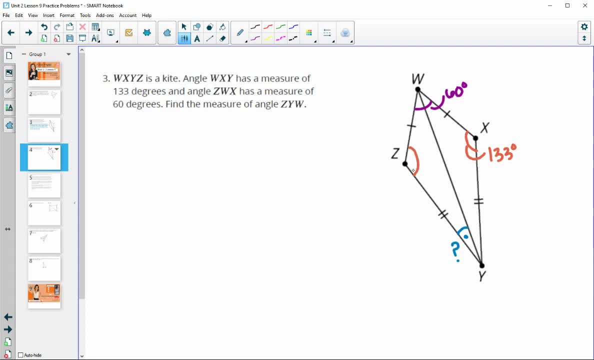 congruent. so Z would be a corresponding angle with X. so we know that Z would also be 133 degrees. and so now we can see that we've got three of the angles in the kite that we know, and we know that the total degrees in a 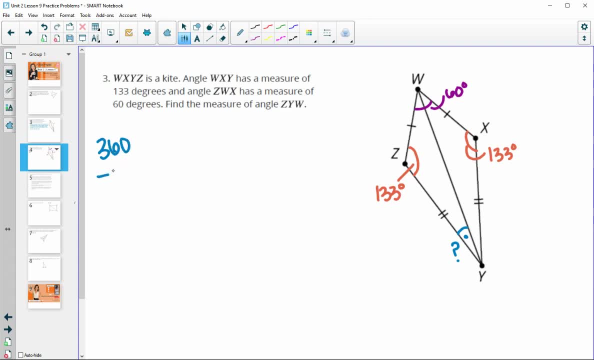 quadrilateral is 360. so if we take 360 and subtract off these three angles from the total, we will have the leftover of 35 degrees. So we're going to get 34 degrees for this larger angle down here. so for this one, and then, since these two triangles are congruent, these two angles are the same. 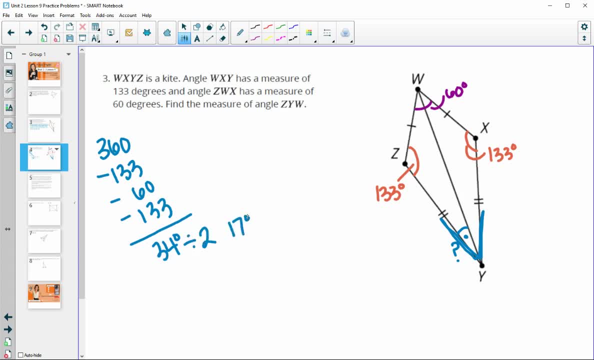 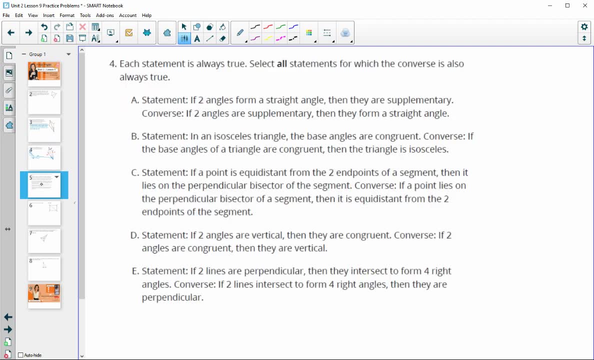 so we'll take this 34 and divide it by two to get 17 degrees for this little angle here. Number four tells us that the statement in each case is true. so we're going to have a statement which is true. Then it's going to do the converse for us, which is when we flip the end and the beginning around. 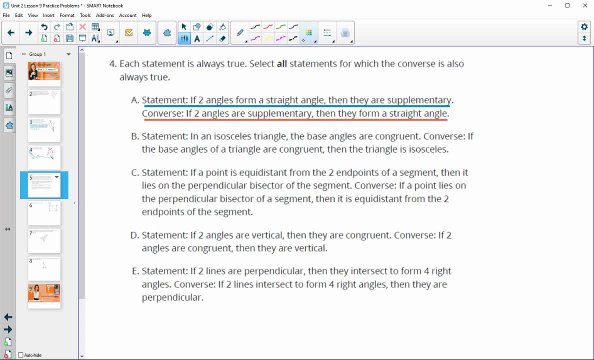 and we're supposed to decide if the converse of each statement is also true. So in A it says: if two angles are supplementary, then they form a straight angle, because it is true that a straight angle split into two angles will always be supplementary, so this will always total 180. 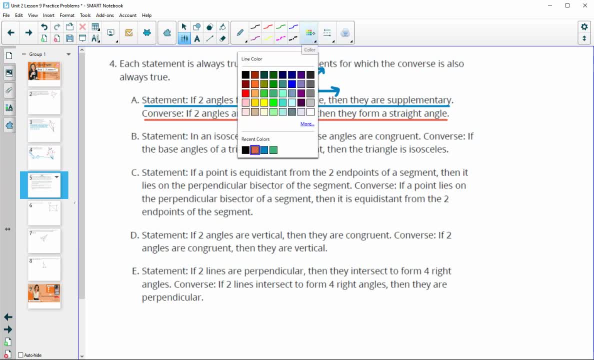 But is it true that if we know that the angles are supplementary, they form a straight angle, and that is going to be false. so let me do a counter example here. so if we have a 110 degree angle here, then we could have a 70 degree angle. 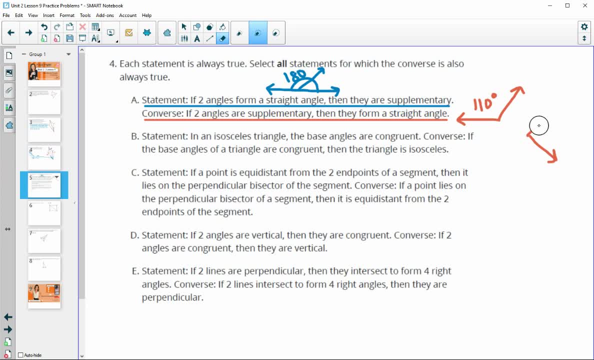 Oops, that doesn't quite look like 70, looks more like 90. Then we could have a 70 degree angle here. those two angles are definitely supplementary. They add to 180, but they um are not. they do not make a straight angle. 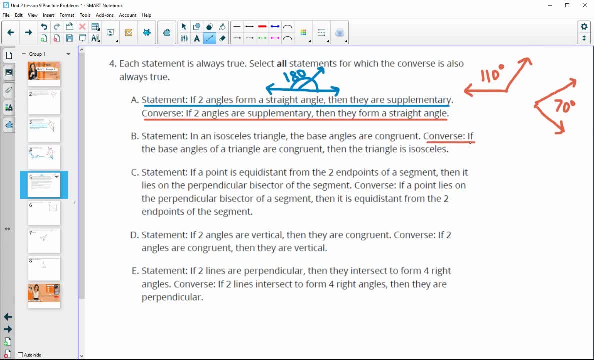 Second one: if the base angles of a triangle are congruent, then the triangle is isosceles. This is the base angle theorem. so if we know that this angle is congruent to this one, then we know that the sides across are congruent. 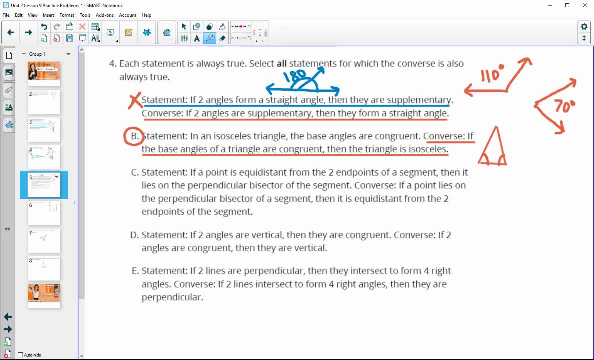 so that is true. so this one is false. that's true, um. the third one says: if a point lies on the perpendicular bisector of a segment, then it is equidistant from the two end points of the segment. so if i have a segment and they have the perpendicular bisector, 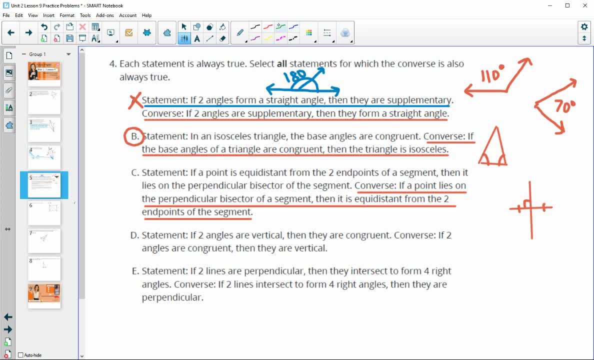 so we know that this is a 90 degree angle and these are congruent, then any point on here is going to be equidistant from the ends. we know that to be true, so that one is true. fourth one: if two angles are congruent, then they are vertical. so let's remember. 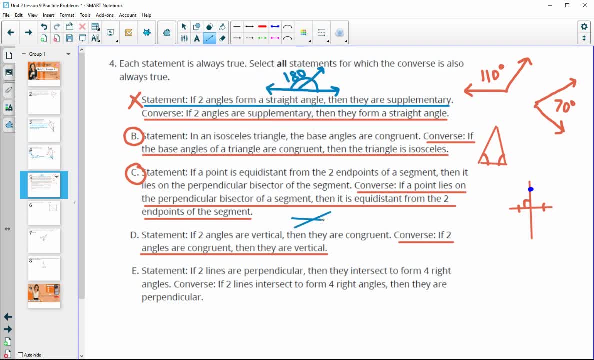 um, that vertical angle. so the original statement is going to be that vertical angles are congruent. so anytime you have two straight lines crossing here, then the angles across from each other are called vertical angles and they are congruent. um, so if we switch that, if two angles are, 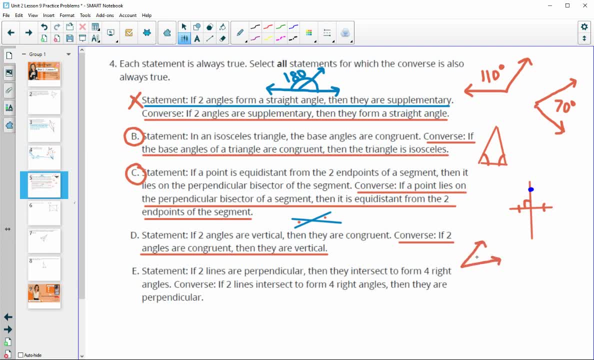 congruent, do they have to be vertical? and that's false. so we could have um like a 30 degree angle here, and then we could have a 30 degree angle here. they are definitely not vertical because they don't share um even the same vertex, so that would be a counter example to this. so this is 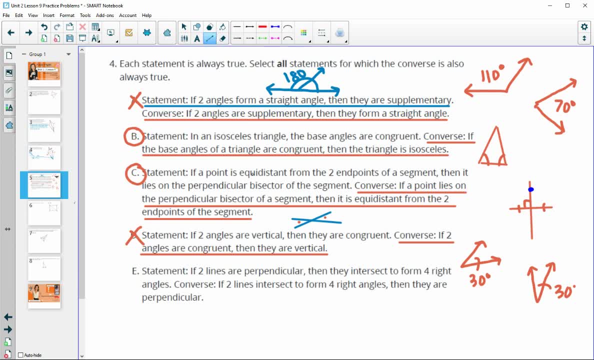 false. and then the final one says that if two lines intersect to form right angles, then they are perpendicular, and we'll will demonstrate that here. that's a good thing, but I'm going to just never pass through that and i'm gonna give you you, we're going to hash this over. they would be. 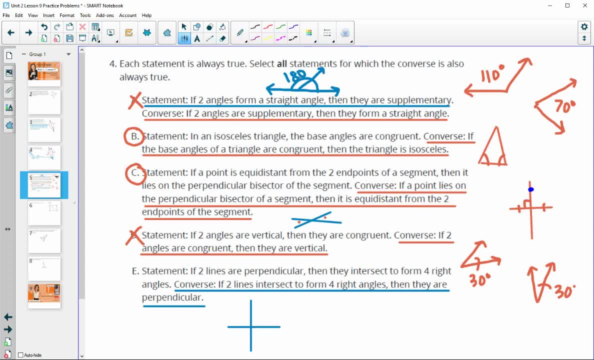 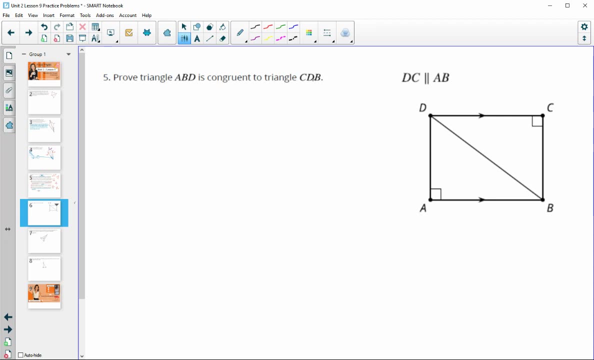 know that that is true because perpendicular lines meet to form right angles. So if we've got four right angles here, then these are definitely perpendicular angles, or sorry, perpendicular lines. Number five prove that triangle ABD is congruent to triangle CDB. 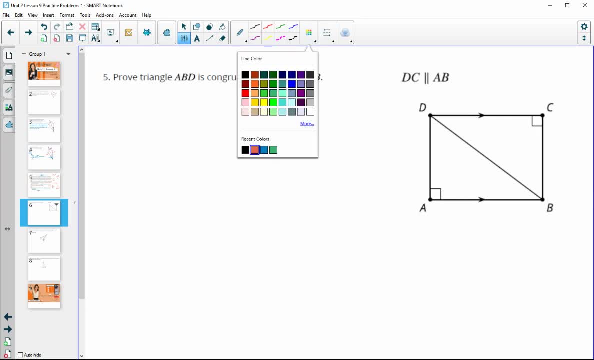 So let's take a look at what they're giving us and come up with a plan first. So they're telling us that the lines are parallel and we also see these right angles. So we know that A and C are equal. When we have parallel lines, we can do alternate interior angles, So we know that this. 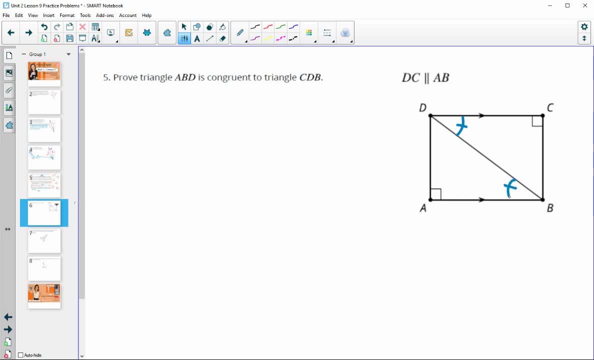 angle is congruent to this angle, And then we can't get that these two parallel lines are congruent to each other, but we can tell that this middle segment is in both triangles. So now what we have in each triangle is this Side, this angle and this angle. So that doesn't give us angle, side angle, because we don't have. 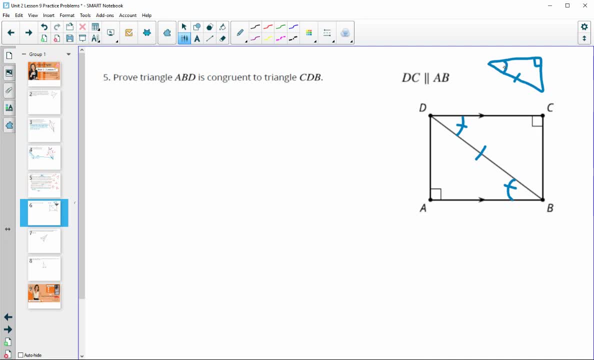 the included side, but we do have two of the angles, So we should be able. we can then conclude that this third angle- okay, so this one here is congruent to this one, because the sum of every triangle is 180.. So if we subtract this, these same two measures from 180 here, we'll get the 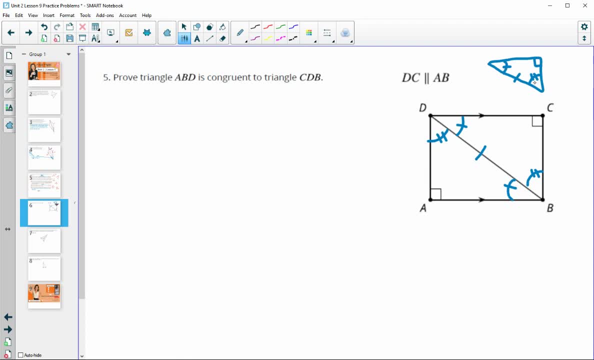 same amount as we would in this triangle, In which case then we have angle side angle to prove that the two triangles are congruent. So that's the plan. Then you just got to write it out. So we could just say angle A is congruent to. 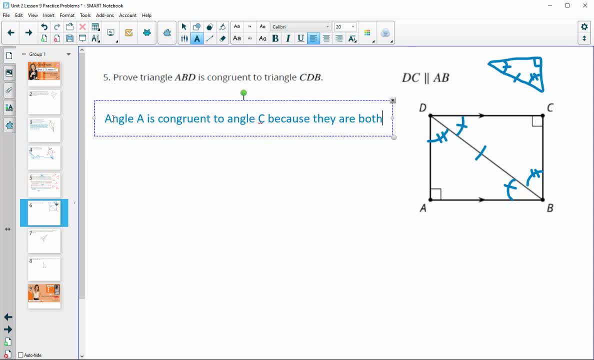 angle C because they are both right angles. Then we said: angle ABD is congruent to angle CBB because they are alternate interior angles formed by two parallel lines. BD is congruent to DB because it is the same segment in both triangles and then by triangle sum theorem we can conclude that angle ADB is congruent to. 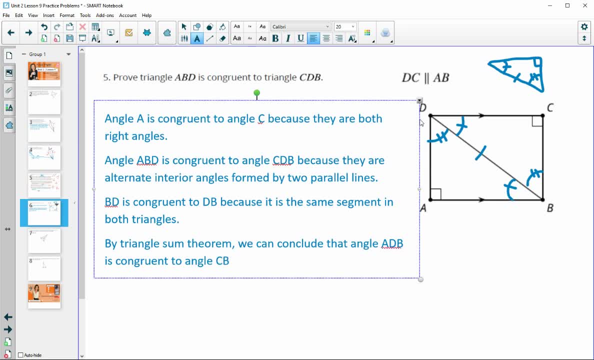 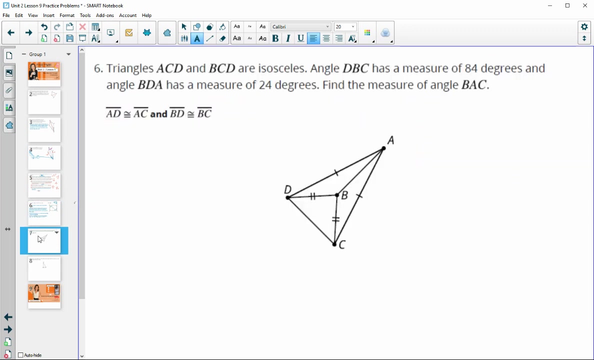 angle CBD. therefore, triangle ABD is congruent to triangle CDB by angle side angle congruent triangle: congruence number six. we've got to trying to isosceles triangles that are marked angle DBC has a measure of 84 degrees, so this angle here is 84 and angle BDA is 24, so BDA is 24 degrees. find: 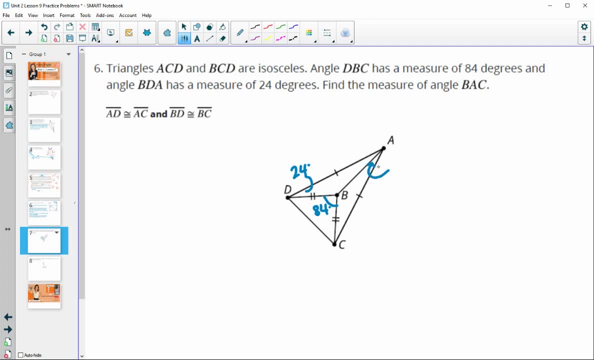 the measure of BAC. so we want this little angle here over. so we've got isosceles triangles and we're looking at angles, so we probably want to be looking at base angle theorem. so in this little isosceles triangle down here we've got the 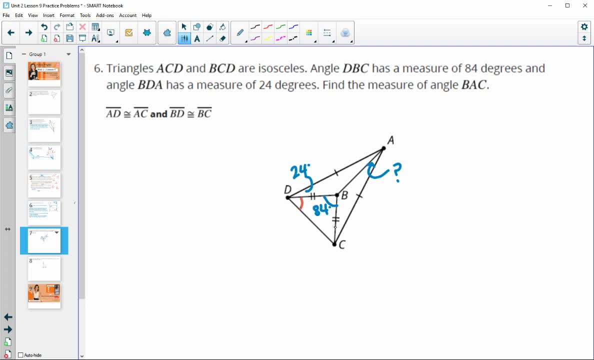 vertex angle and then we know that these two angles are congruent. so if we do 180 and we subtract off that 84, we know we have 96 degrees left over for those two angles. they're exactly the same size, so we'll just divide by two and get that each of those. 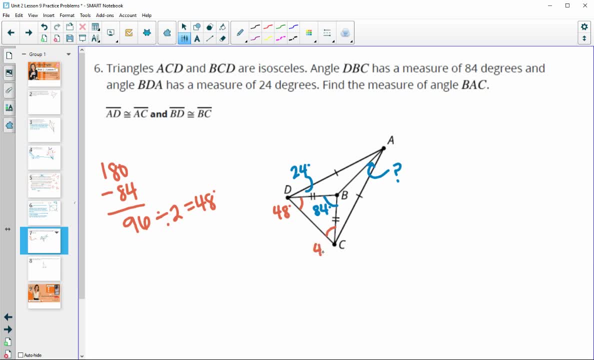 angles are 48 degrees, so then we ultimately need to get this angle up here. but now we can kind of see that we know this whole angle. if we just total those together we would get 72 degrees, and since this big triangle is an isosceles triangle, this one here is also 72 degrees. 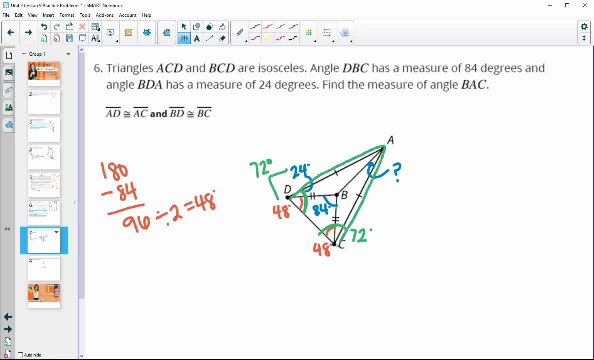 and this whole triangle would total 180. so we can do 180 minus 72 minus 72, which gives us 36 degrees for this full angle up here. and then we only want half of that. so we're going to take this 36 and divide it by 2 to get 18 degrees for this.